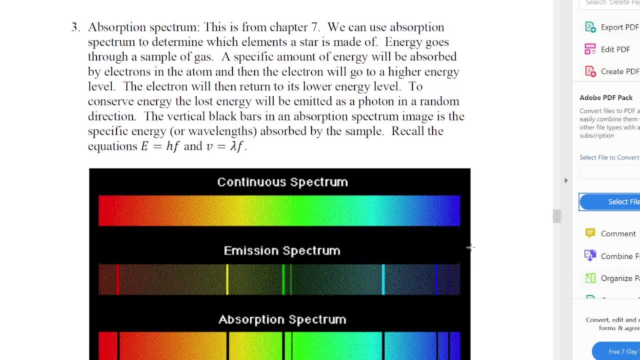 number three: the absorption spectrum. so this is from chapter seven. we can use the absorption spectrum to determine which elements a star is made of. energy goes through a sample of gas or electromagnetic waves. okay, a specific amount of energy will be absorbed by electrons in the atom and then the electron will go to a higher energy level. then the electron will then return. 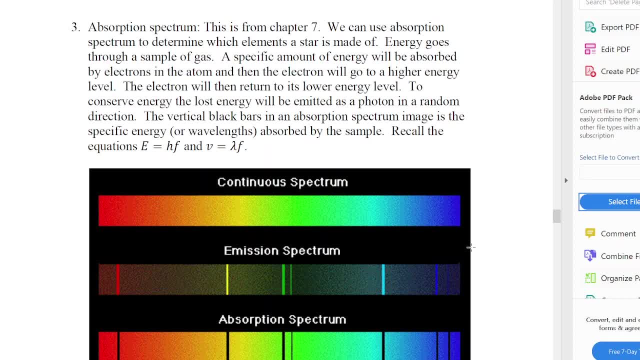 to a slower energy level to conserve energy. the lost energy will be emitted as a photon in a random direction and the vertical black bar is in an absorption spectrum. and the black bar is in an absorption spectrum image is the specific energy or wavelengths absorbed by the sample. 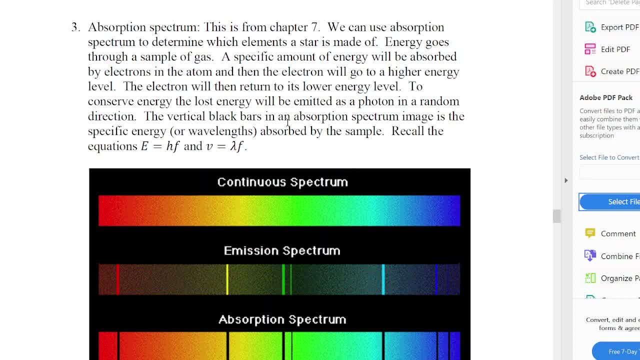 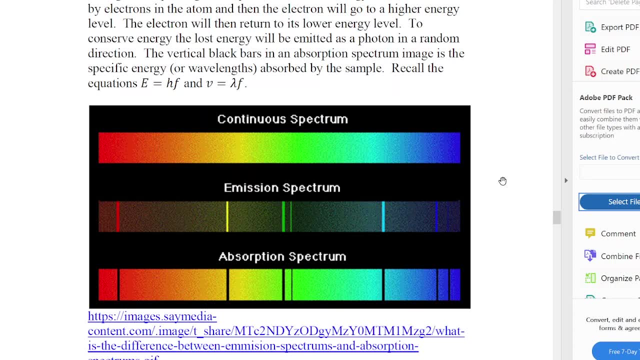 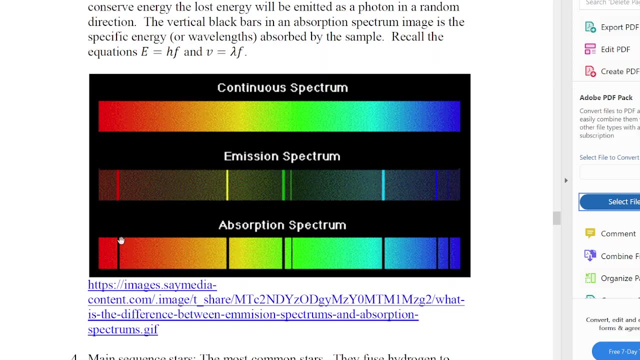 okay, so recall the equations: e equals hf and v equals lambda f. okay, and also, uh, review topic seven. so this is the absorption spectrum, the emission spectrum and the continuous spectrum. so remember, the absorption spectrum and emission spectrum is like the fingerprints of an atom. okay, so this is the absorption spectrum, the emission spectrum and the continuous spectrum. 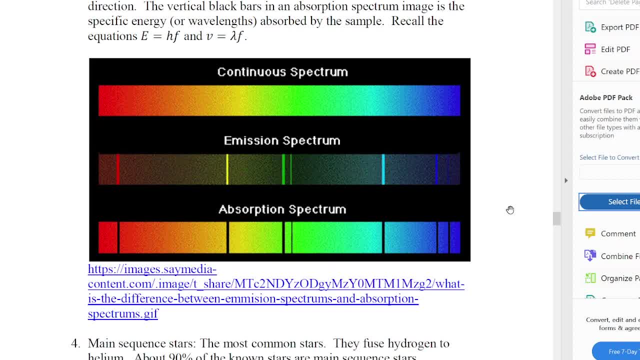 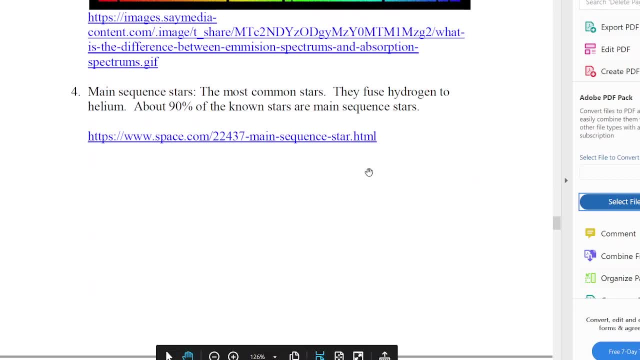 uh of an element. hydrogen is different than helium. helium is different than lithium. you get the point number four: main sequence stars. okay, these are the most common stars. they fuse hydrogen to helium and about 90 percent of the known stars are main sequence stars. so our sun, 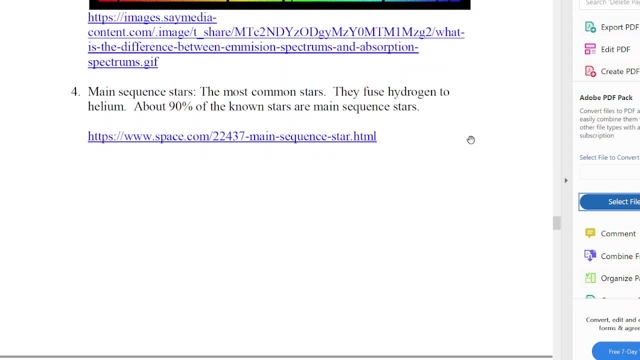 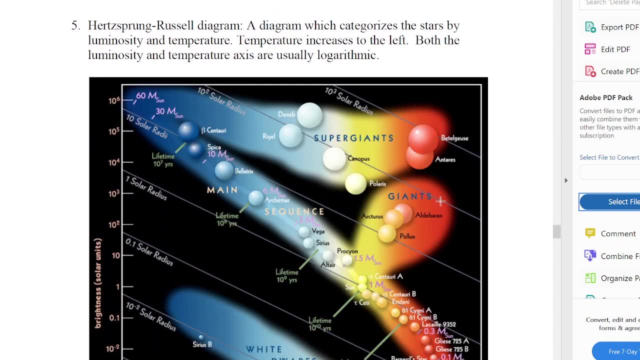 which is a star, is a main sequence star. for more information you can go on this website, okay, the the hertz sprung russell diagram is a diagram which categorizes the stars by luminosity and temperature. temperature increases to the left. both the luminosity and temperature axis are usually 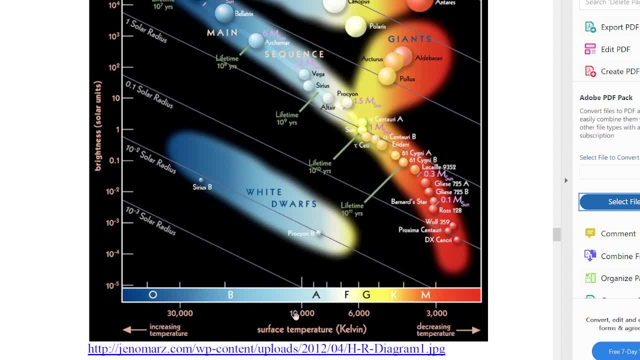 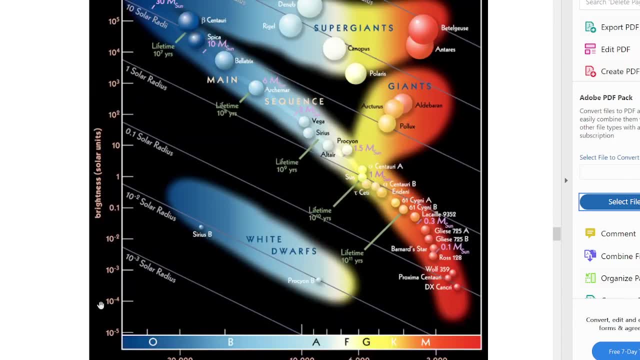 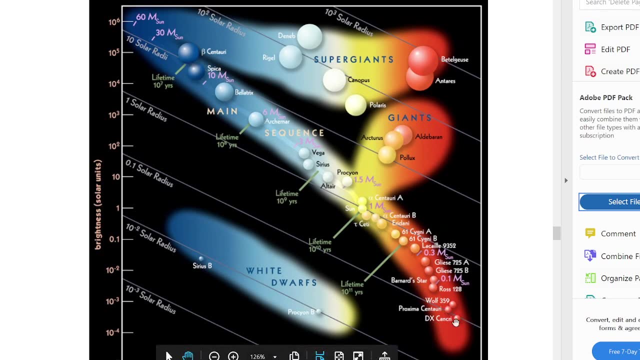 logarithmic. so take a look at this graph: temperature increases to the left and is logarithmic, and the brightness is increases as you go up and that's logarithmic, and see this line or this curve. they call this the main sequence. you can see it says main sequence. this is the main sequence of. 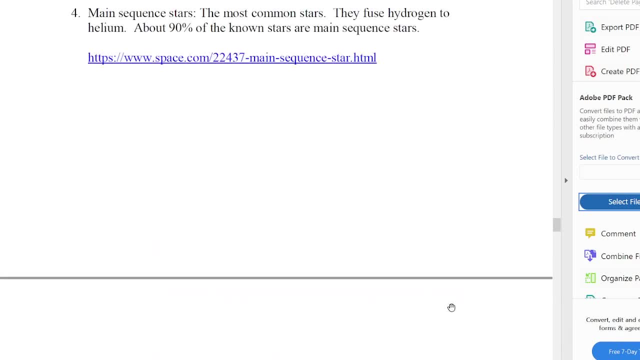 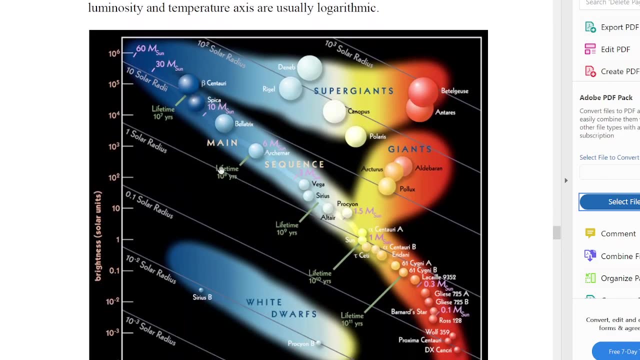 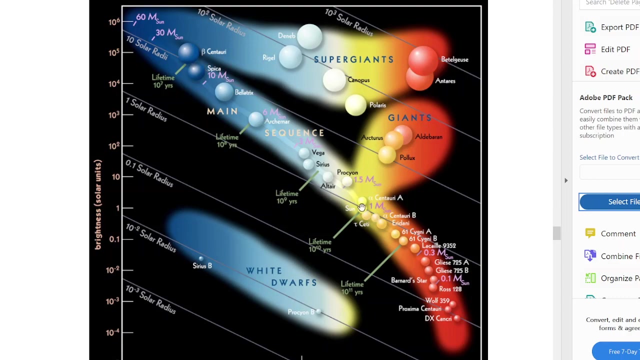 stars. this is where most of the stars are, so remember the meaning of main sequence stars. about 90 of the known stars are main sequence stars, so about 90 of them are on this curve. okay, the sun is right here. it's a main sequence star, okay, so spectroscopic. 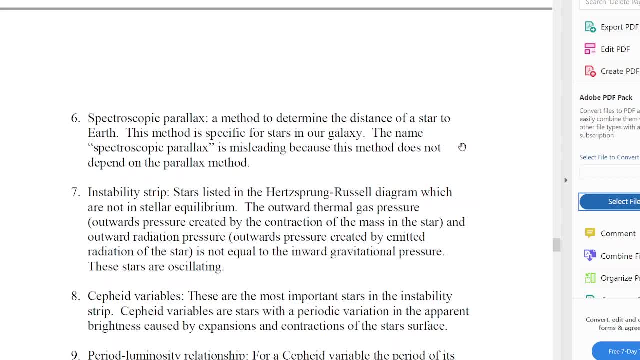 parallax is a method to determine the distance of a star to earth, and this method is specific for stars in our galaxy. the name spectroscopic parallax is misleading because this method does not depend on the parallax method instability strip. these are stars listed in the hertz sprung. 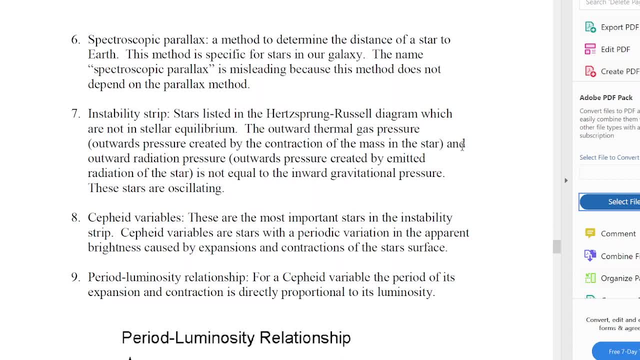 russell diagram, which are not in stellar equilibrium. the outward thermal gas pressure, which is the outwards pressure created by the contraction of the mass of the star, and the outward radiation pressure, which is the outwards pressure created by emitted radiation of the star, is not equal to the inward gravitational pressure. so these stars are: 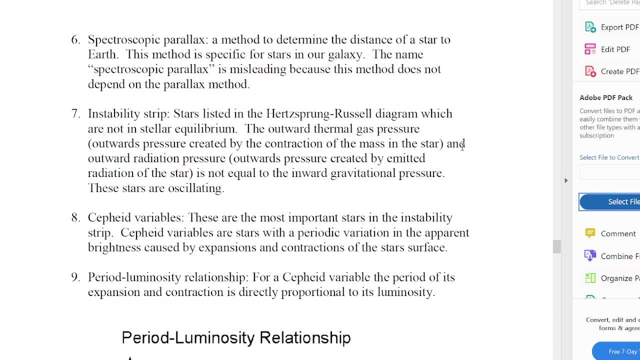 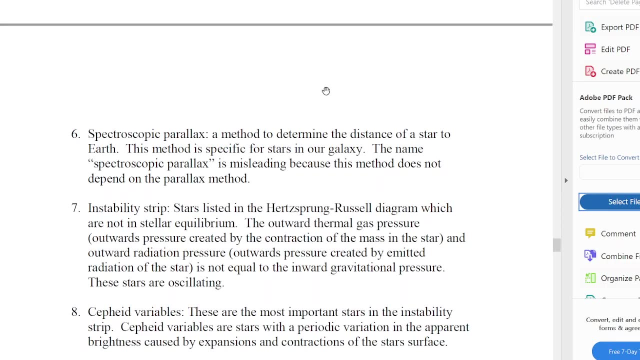 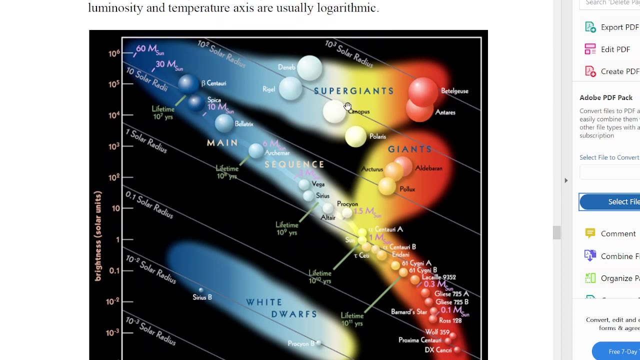 oscillating. think about the volume of the star getting bigger and smaller, bigger and smaller, so it's like a heartbeat. it's just oscillating. so it's definitely not in stellar equilibrium. so could we find the stellar, sorry, can we find the instability strip here? that's, these giants and these super giants here. these are not in stellar. 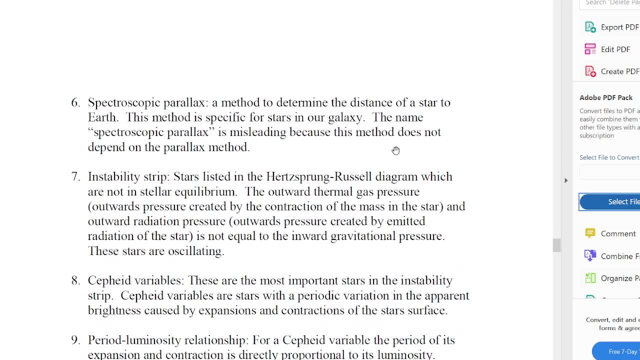 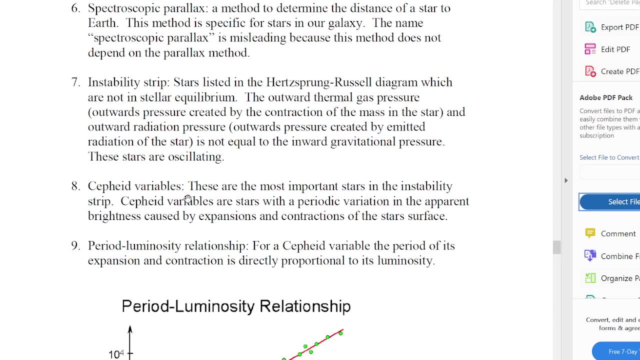 equilibrium. okay, that's the instability strip sephite stars. these are the most important stars in the instability strip. sephite star, sorry. seppheed variables are 외국의 língu, Kevinclockwise의 peppers, kookal ference. of the more important stars are stars with die mandatory cases. sephide variable are stars with dashed failures. this is the dominant. 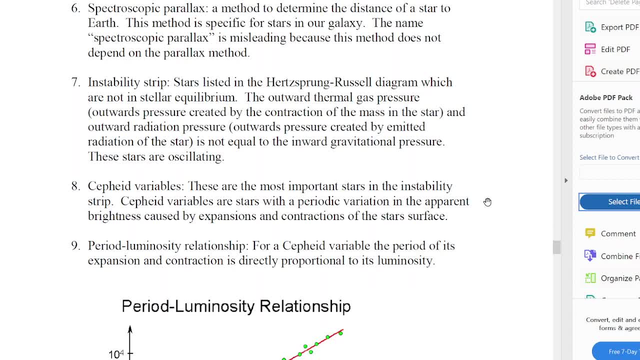 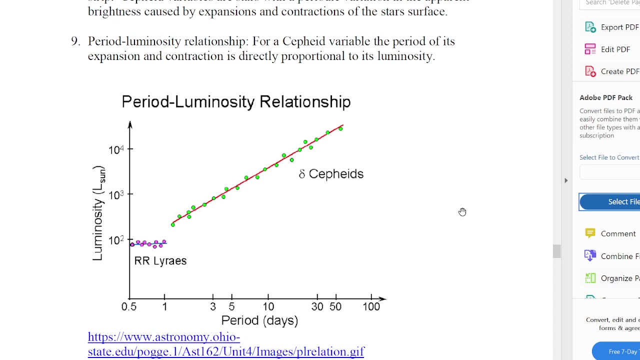 a periodic variation in the apparent brightness caused by expansions and contractions of the star's surface. so remember what i said: the star is like beating um. the gravitational pressure inward is not equal to the thermal and radiation pressure outward. number nine: period luminosity relationship for a cepheid, very variable the period of its expansion. 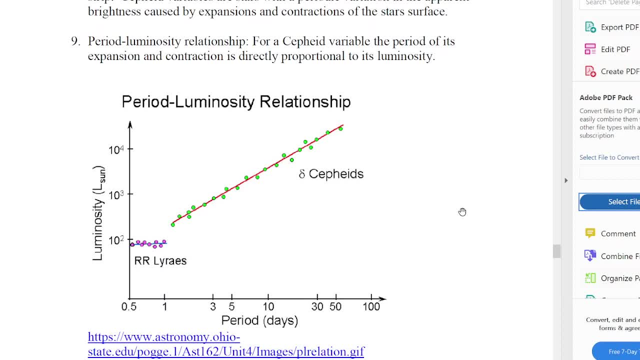 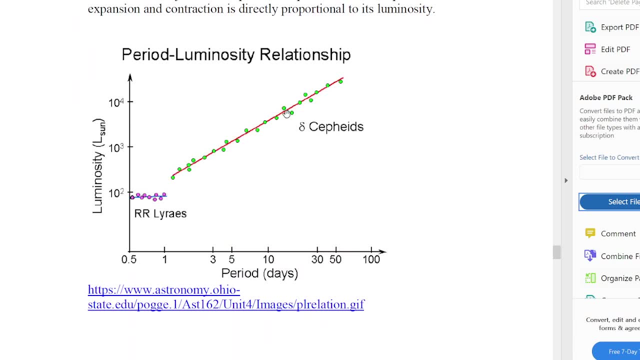 and contraction is directly proportional to its luminosity. so remember this is only for a cepheid variable star, okay, and you can see there's a nice relationship here. you see, period here is not linear, looks logarithmic, luminosity looks logarithmic. so as the period increases, the luminosity increases. remember this is not the period around. 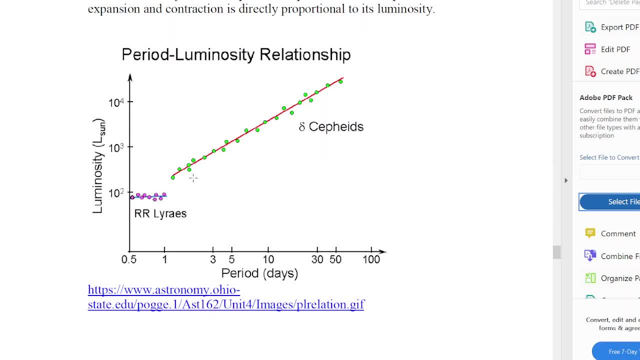 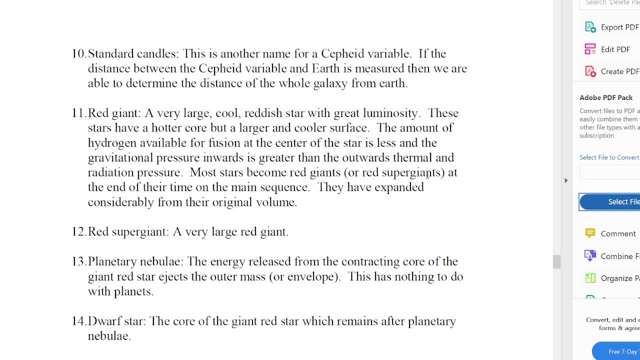 like a planet around a star. this is the period that the star itself oscillates because of its non-stellar equilibrium. number 10 standard candles. this is another name for a cepheid variable. if the distance between the cepheid variable and earth is measured, then we are able to determine the distance of the whole galaxy from earth. 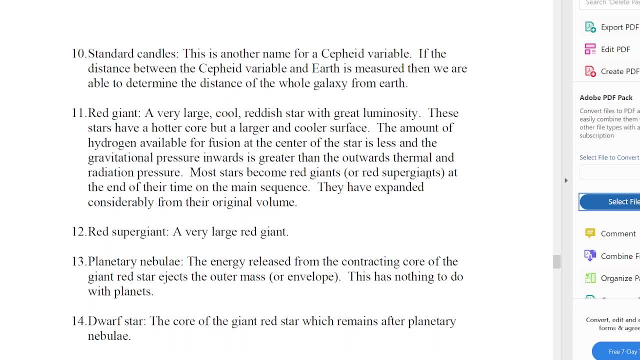 number 11, red giant. number 12, a very large, cool reddish star with great luminosity. these stars have a hotter core but a larger and cooler surface. the amount of hydrogen available for fusion at the center of the star is less and the gravitational pressure inwards is greater than the. 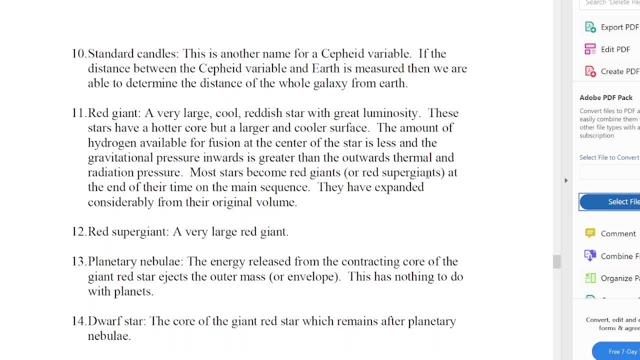 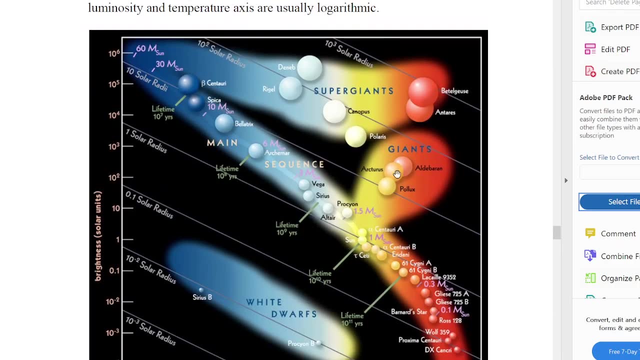 outwards thermal and radiation pressure. most stars become red giants or red super giants at the end of their time. on the main sequence, they have expanded considerably from their original long. So where are the red giants? They're here Up here. Red giants and red supergiants- okay, These are definitely unstable. A red supergiant is a very large red giant. Planetary nebulae is. the energy released from the contracting core of the red giant star Ejects the outer master envelope. So this has nothing to do with planets, even though it's called planetary nebulae. 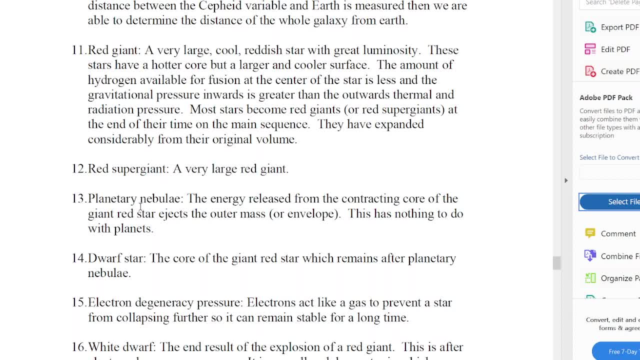 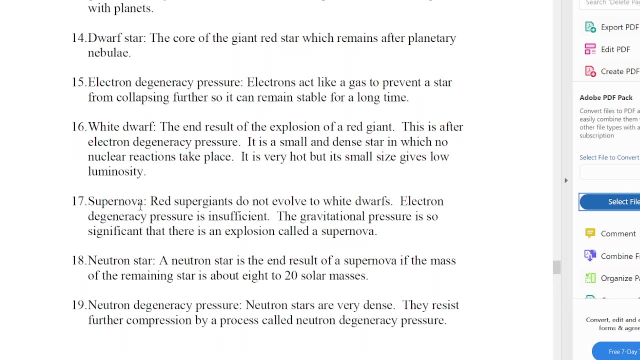 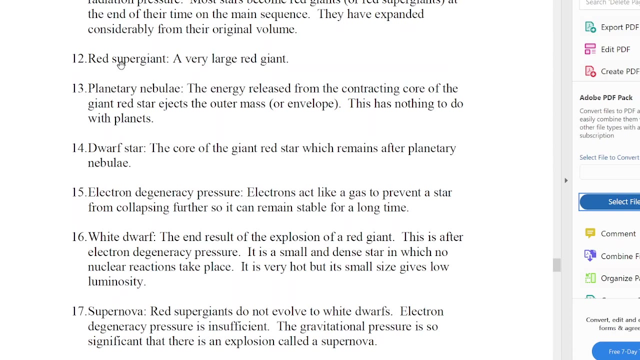 So it's like a sphere losing its shell, okay, Like there's an explosion and the outer mass of that star leaves. Number 14, dwarf star. This is the core of the giant red star which remains after planetary nebulae. So first there's a red giant or a red supergiant, Then there's planetary nebulae And finally there's a dwarf star. 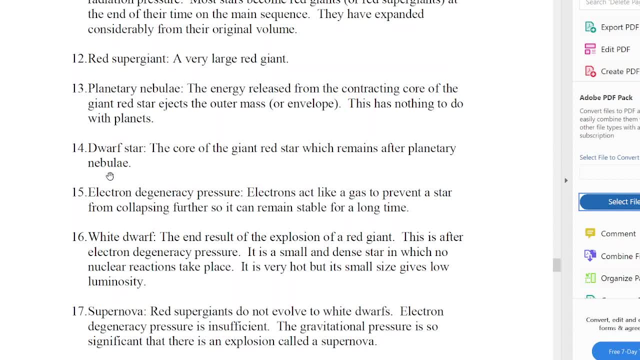 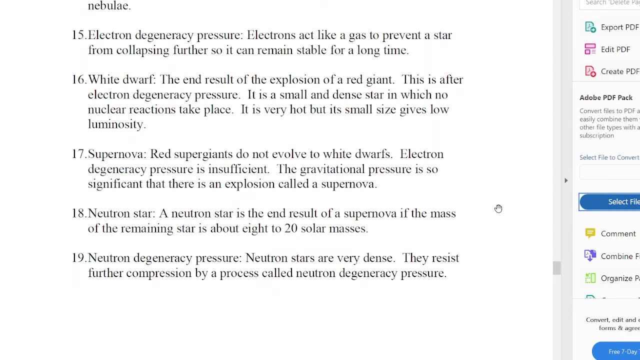 15, electron degeneracy pressure. This is electron degeneracy pressure. This is electron degeneracy pressure. This is electrons acting like a gas to prevent a star from collapsing further so it can remain stable for a long time. 16, white dwarf. This is the end result of the explosion of a red giant. This is after electron degeneracy pressure. 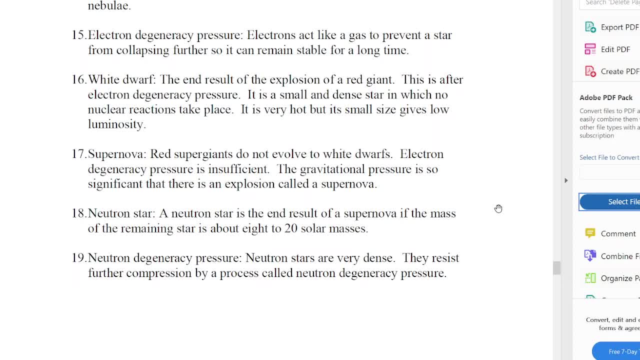 It is a small and dense star in which no nuclear reactions take place. It is very hot, but its small size gives it a lot of energy. It is a small and dense star in which no nuclear reactions take place. It is a small and dense star in which no nuclear reactions take place. 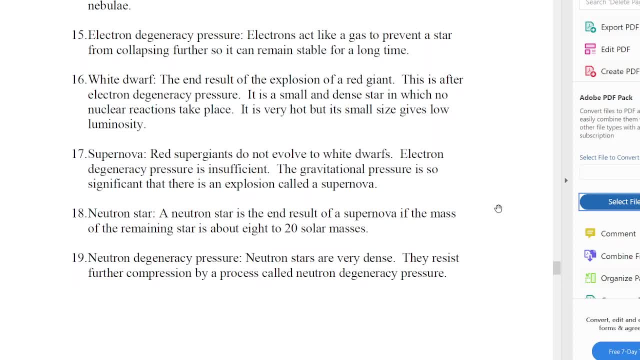 This is electron degeneracy. pressure pressure is insufficient and the gravitational pressure is so significant that there is an explosion called a supernova Number 18, neutron star. It's a star at the end result of a supernova. if the mass of the remaining star is about 8 to 20 solar masses, A neutron star is very dense. 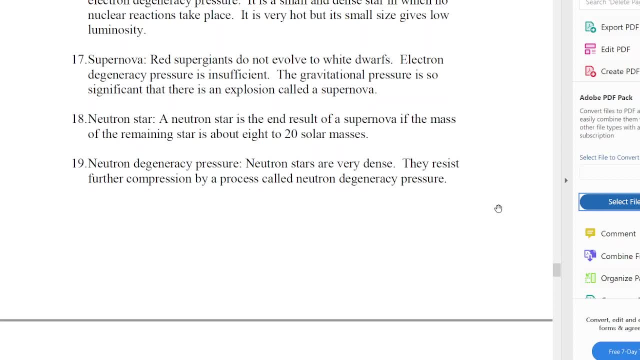 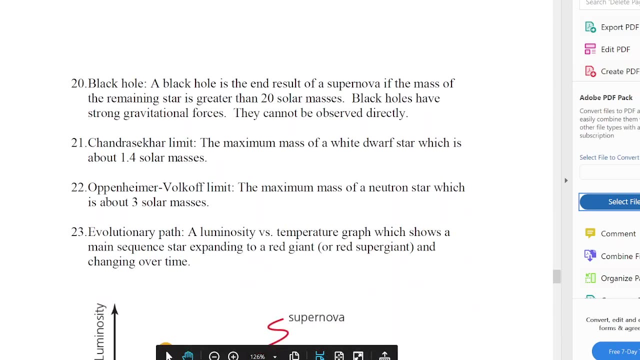 It's a neutron degeneracy pressure. This is neutron stars which are very dense and they resist further compression by a process called neutron degeneracy pressure. Number 20, black hole. A black hole is the end result of a supernova. if the mass of the remaining star is greater than 20 solar masses, Black holes have. 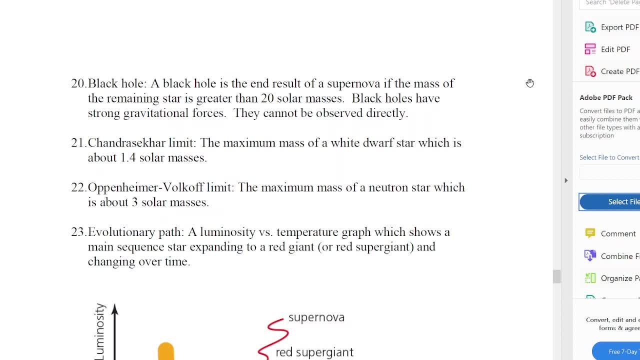 strong gravitational forces and they cannot be absorbed. Number 20, Chandrasekhar limit is the maximum mass of a white dwarf star, which has about 1.4 solar masses. 22, Oppenheimer-Volkoff limit is the maximum mass of a neutron star, which is about 3 solar. 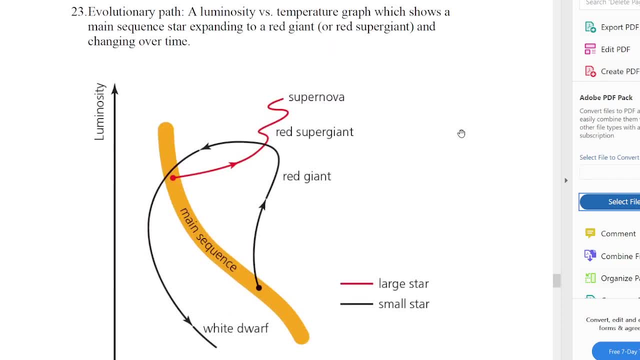 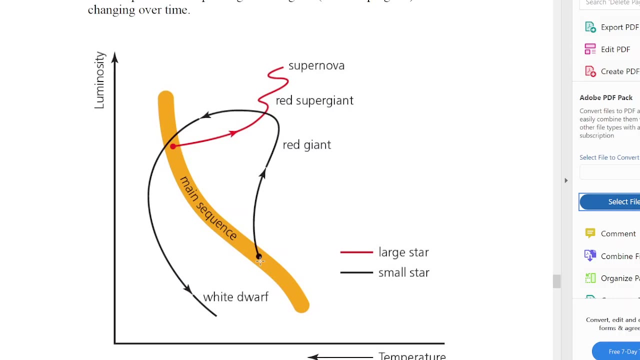 masses. 23 is the evolutionary path. This is a luminosity of a neutron star which is about 3 solar masses. 24, Peltier limit is the minimum mass of a neutron star, which is about 3 solar masses. The. 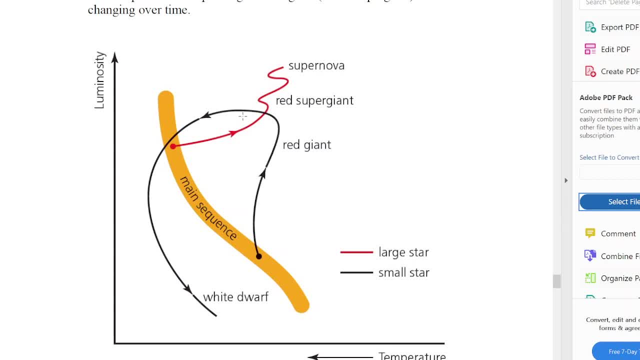 estimated oblique velocity of a neutron star is around 22,000 kilometers per second. The average velocity of a black hole star is about 22,000 kilometers per second, The average velocity of a bright. so there's a lot going on here. now look at this larger star. 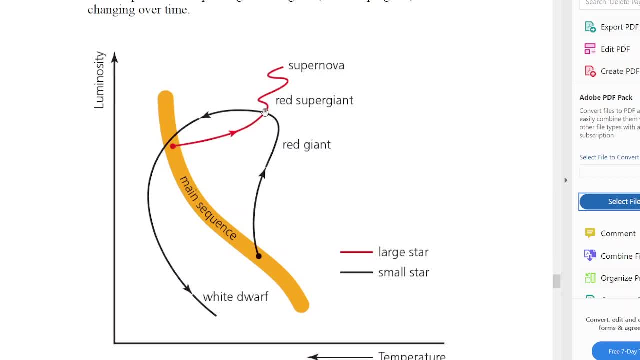 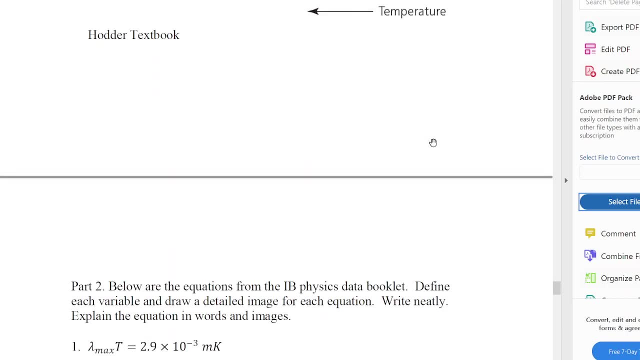 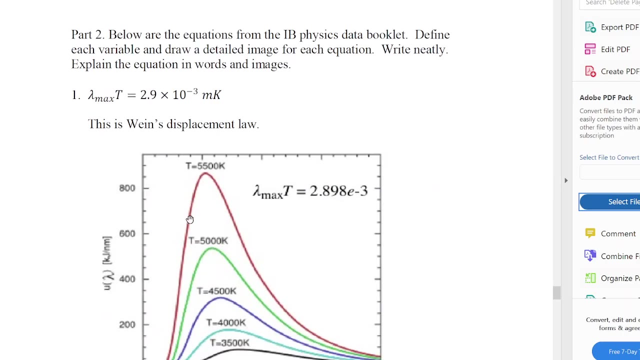 its temperature decreases as its luminosity is increasing, and then here it's kind of oscillating with its luminosity and temperature. I got this image from the Hodder textbook. it's a great textbook. please read it. part 2, below are the equations from the IB physics data booklet. 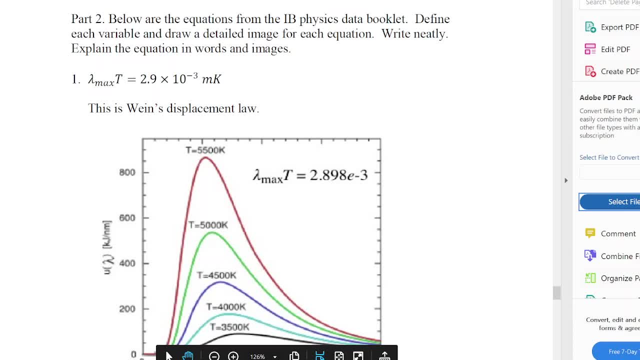 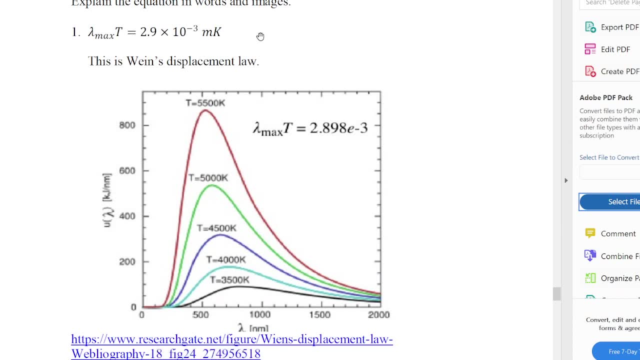 so let's talk about these equations. number 1: lambda max times t equals a constant which is 2.9 times 10 to the minus 3 meters Kelvin. so the right hand side doesn't change. it says on the left hand side: if the temperature of the black body increases, 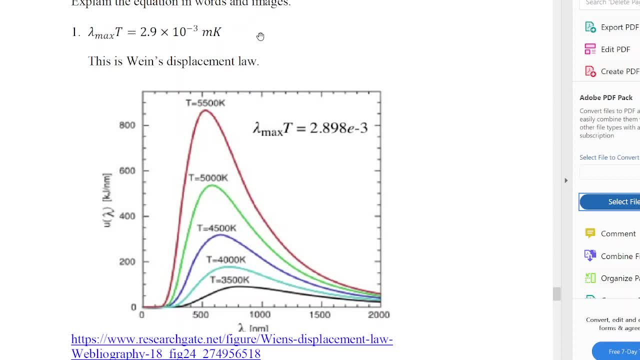 then the maximum wavelength emitted by the black body decreases. it's an inversely proportional relationship. so you can see, at 5500 Kelvin a black body is emitting all different kinds of wavelengths except these super short ones here, and the maximum wavelength emitted is given by this equation. 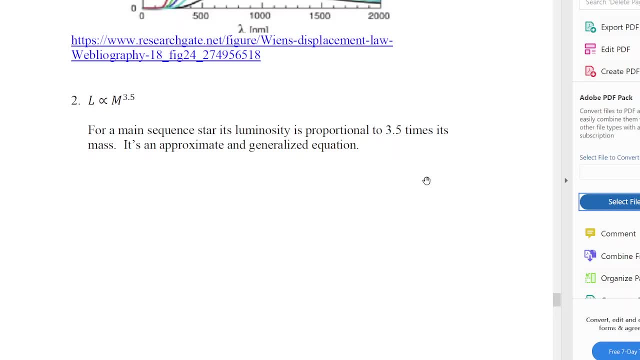 equation 2 is super important. luminosity is proportional to m to the 3.5. so it says: the mass of a star to the 3.5 power gives a maximum wavelength. of m to the 3.5 power gives us the luminosity.